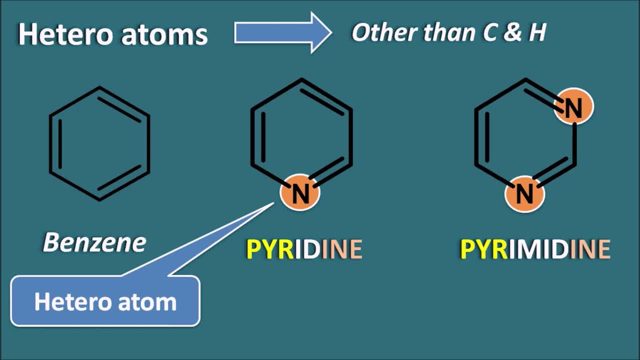 rings are having the same prefix, pyr, and they're having the same suffix, ein. So we can remember the hetero cyclic rings by using few of the prefixes and by using few of the suffixes. So in this video we will go with the hetero cyclic rings- how we can remember- and any possible suffixes as well. 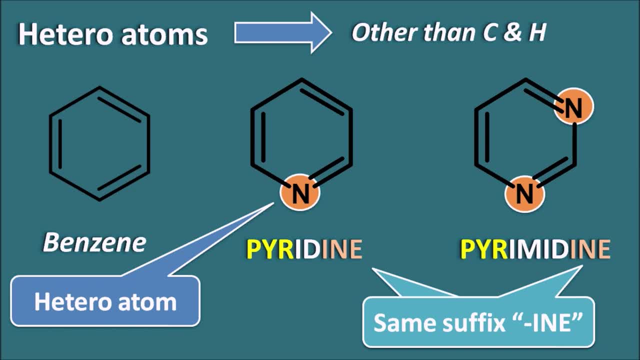 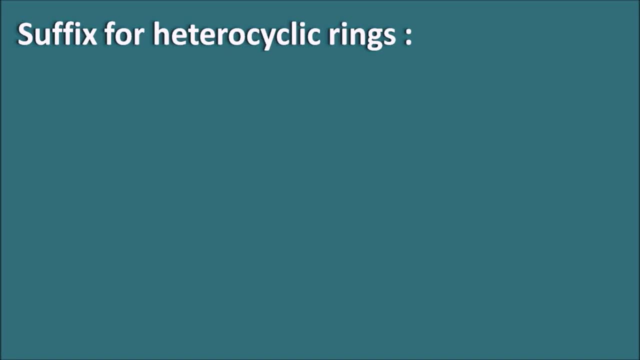 as the prefixes present for the hetero cyclic rings. Suffix for the hetero cyclic rings. So we can have a a broad hetero cyclic nomenclature. but here we are going to see how easily we can remember this hetero cyclic rings by using few of the suffixes. The suffix for the hetero cyclic rings can be: 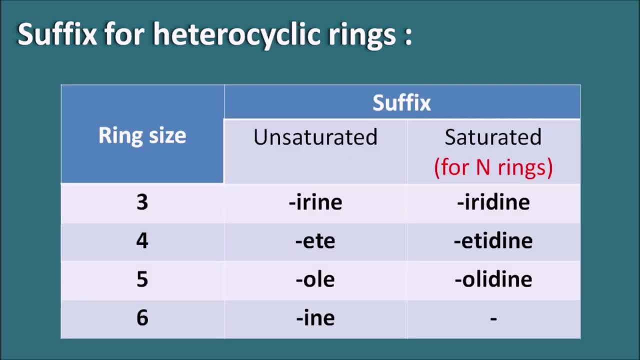 given based on the ring size. What is the ring size and what is the suffix if it is unsaturated and if it is saturated? But here we have shown the suffixes for the saturated rings which are having the nitrogen. So if the ring size is 3 and if it is unsaturated, that is the iron and if it is. 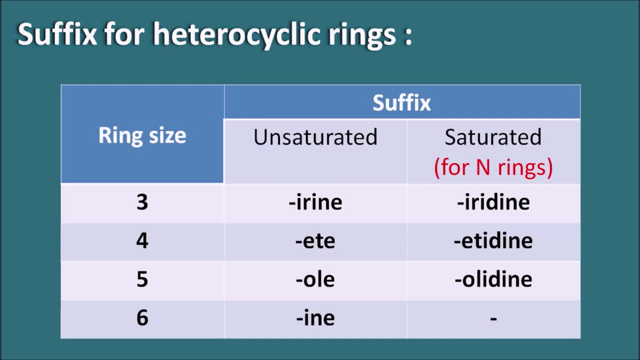 saturated and nitrogen containing ring, it is the iridine, Similarly four, that is it, and saturated etidine, Five all and if it is saturated, olvidin and six iron. but there is no suffix for the saturated ring. From the ring size 6 onwards, the saturated rings will not have any a particular. 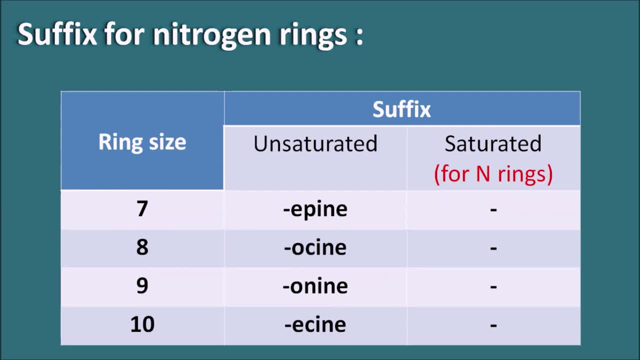 suffix, Similarly the ring size 7.. If it is unsaturated epine but there is no suffix for the saturated, Similarly 8-osin, 9-onin and 10-isin. So if we remember these suffixes we can easily build. what is the name of the heterocyclic? 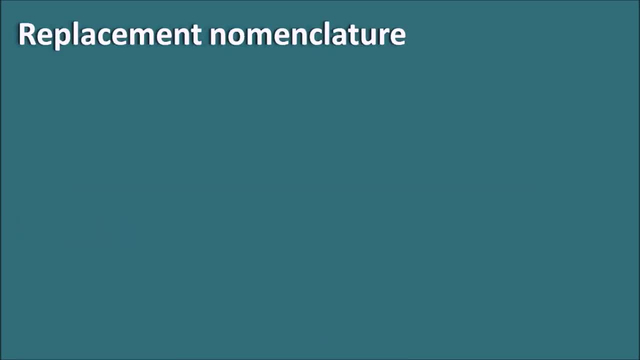 ring system. And another important thing is the replacement nomenclature that we use along with the heterocyclic rings. For example, if nitrogen is there, nitrogen is actually replacing the carbon of the aliphatic ring. So here we can use few of the terms based on the heteroatom. 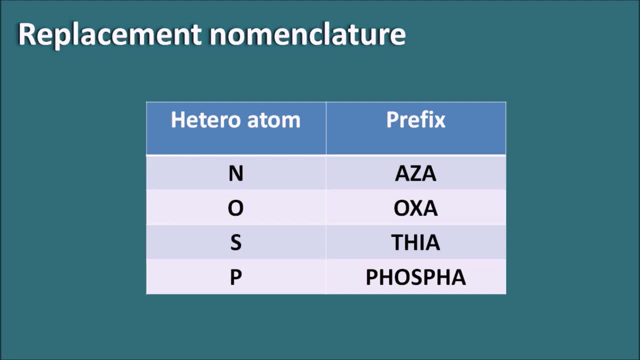 So if nitrogen is there, we can use the prefix aja. If oxen is there, oxa sulpha is there thia and phosphorus as phospha. So in this way any of the heteroatom can be indicated by few of the prefixes. 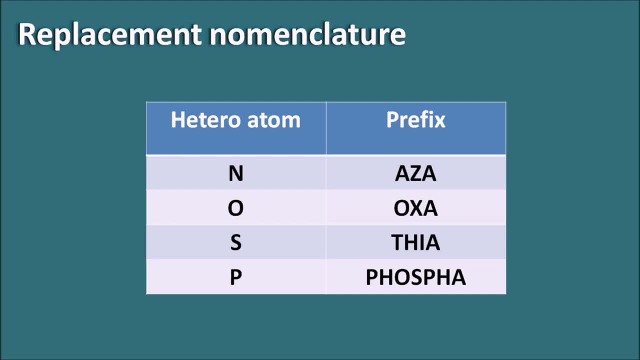 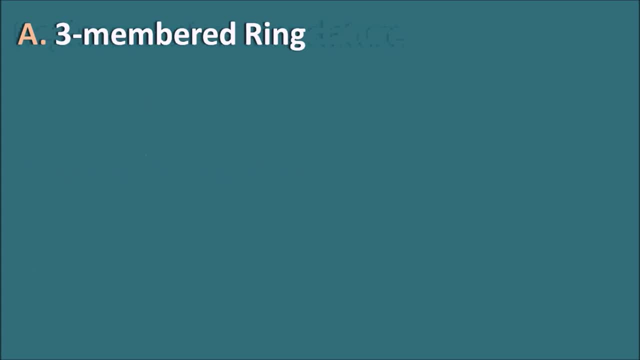 So by using these suffix and prefix, now let us go with the discussion of how easily we can remember the heterocyclic ring systems. So let us start with the first one: three membered ring. So this is simple: Three membered ring containing the nitrogen as the heteroatom. 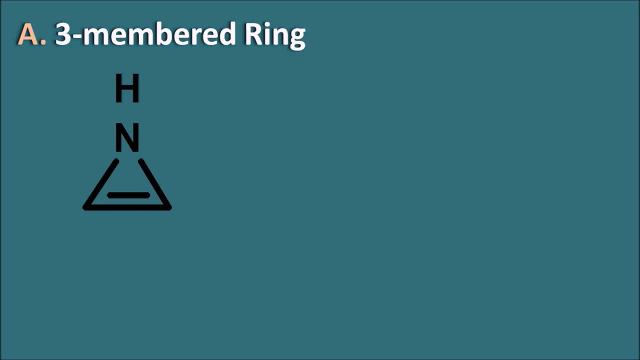 So what is the name of this ring system? Because the nitrogen is present, we have to use the prefix aja plus, Because it is a three membered unsaturated ring system. so the suffix is the irin. So aja plus irin. 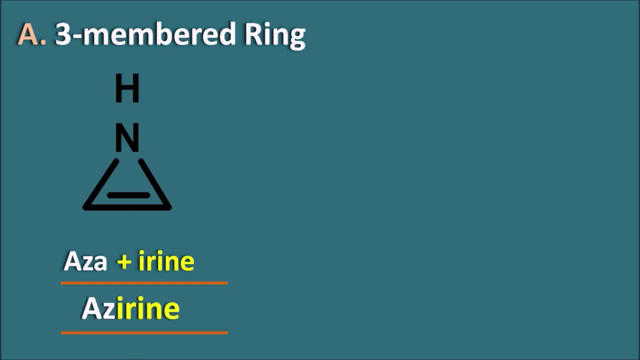 So this is nothing but the egerin. So nitrogen containing heterocyclic ring system which is unsaturated is the egerin, Similarly if it is saturated. So again the prefix is aja plus, whenever it is saturated we can use the suffix iridin. 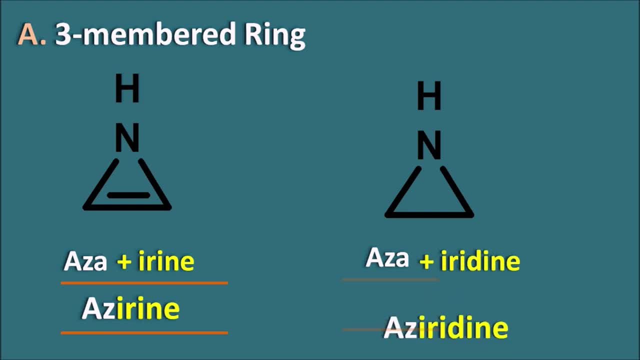 So plus iridin, So aja plus iridin. that is the egerin. Egerin is one of the ring system present in few of the drugs like the thiotepa. Thiotepa is one of an anti-cancer agent which is having the egerin ring system. 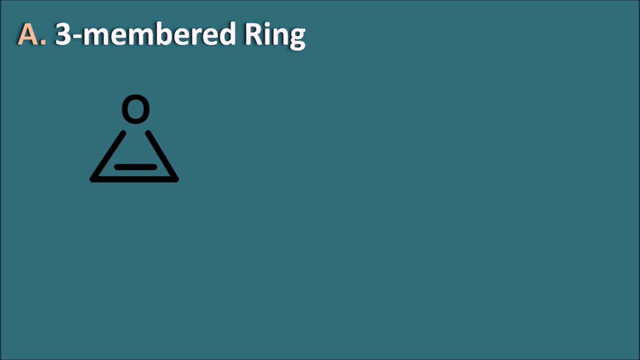 Similarly, another example is the three membered heterocyclic ring with oxen as the heteroatom. So now here we have to use the prefix oxa, So again the prefix is egerin. So again the prefix oxa, plus again the irin. 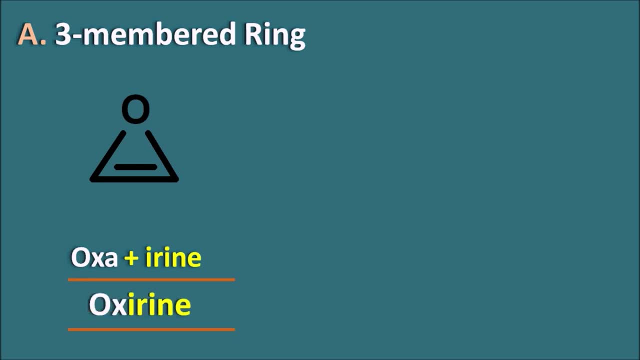 So aja plus irin, it gives the auxerin. Similarly, if it is saturated, then what happens? In the previous example we have seen that the suffix is iridin if it is saturated. but that is a suitable for the nitrogen containing ring systems. 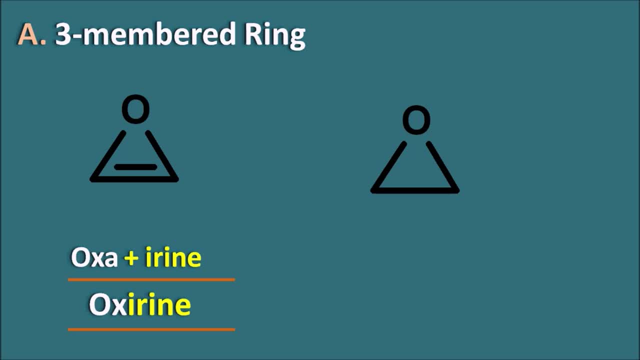 But this ring is not having the nitrogen. this is having the oxygen. When the ring is having heteroatoms other than the nitrogen, we should use a different suffix. So if other than the nitrogen is there, Then if it is saturated we have to use the simple suffix as ane. 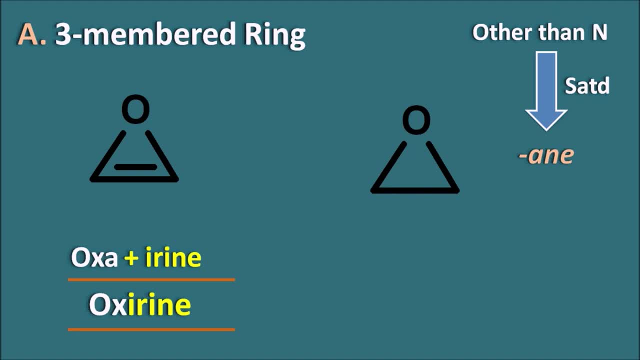 Ane indicates, like all canes, they are saturated. Now this ring system is auxa plus in the irin. we have to replace the ine with the ane, So auxa plus irin. So here ane indicates it is saturated. So auxa plus irin, that is auxerin. 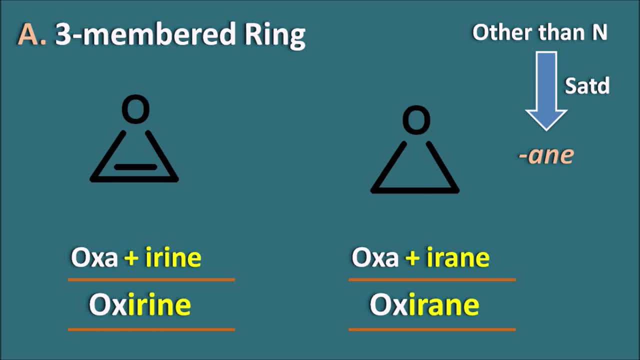 Oxerin is the three membered ring system containing auxin and completely saturated. So this is oxirin. This is oxirin, saturated Similarly with the sulfur. the sulfur can be indicated by thia plus. it is a three member. 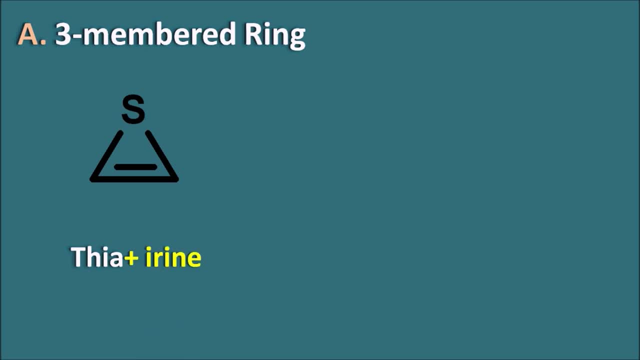 ring system and unsaturated, so that is iron. So that is thia plus iron, thi-iron. Similarly, this ring system here thia plus. if it is saturated, we can write the iron plus an, that is the iron. So thia plus iron, so that is a thi-iron. Now let us go with the four member ring systems. 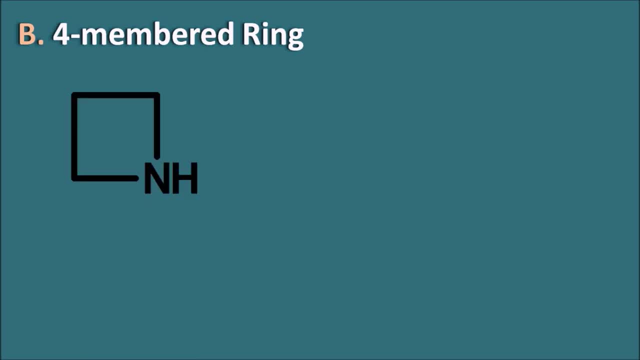 So this is the four member ring system, again containing the nitrogen, and here we are going to discuss few of the heterocyclic ring systems which are more existing in the nature or synthetically. So this is the one of the ring system. So here, what is the name? Again, we have to use the aza. 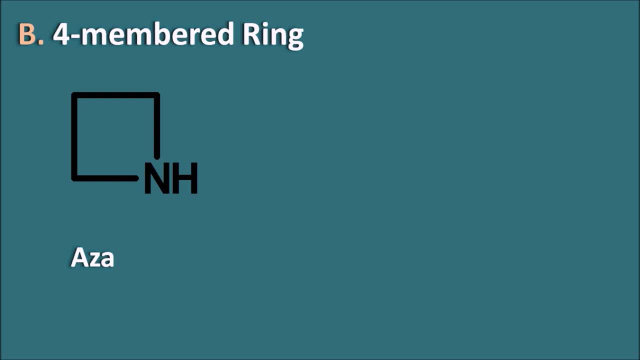 and because it is a four member ring system which is saturated, we have to use the etidine, So aza plus etidine, that is the agitidine. Similarly, another four-membered ring system with auxin, So here we have to use the. 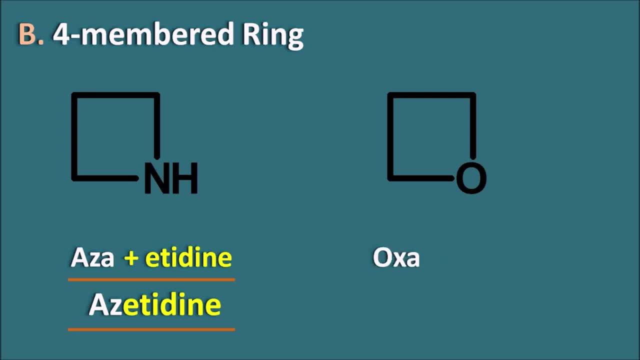 oxa. So here it is the suffix for the unsaturated ring system. But because it is saturated, now the it becomes etane. So oxa plus etane, that is the oxetane And next is the five-membered. 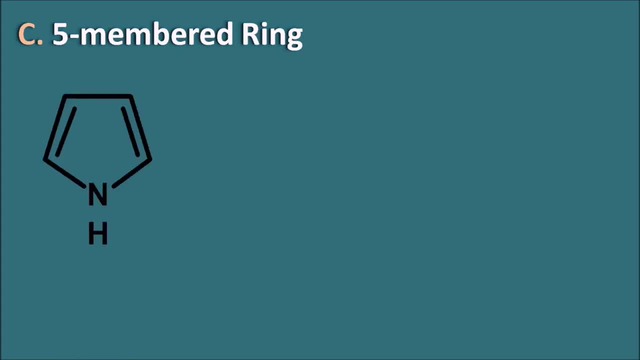 ring systems. So this is one of the five-membered ring system containing the nitrogen, And this is another heterocyclic ring system having auxin, And this is another heterocyclic ring system with the sulfur. Now, what are the names for these three ring systems Here? the first one is the 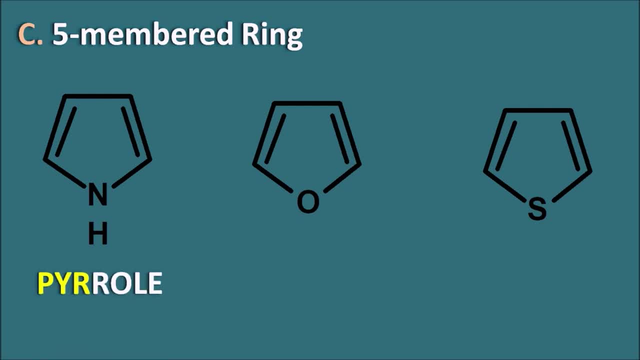 pyrrole. So here pyr is one of the term we are going to use in many of these heterocyclic ring systems And ole is the suffix for a five-membered ring system. So that is a pyr plus ole pyrrole. 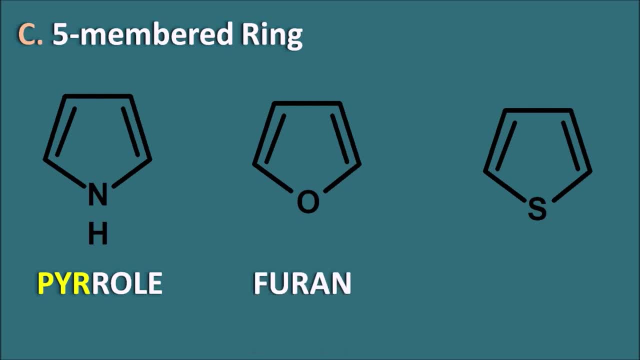 But for second one. the name is the furon. Here we are not using any suffix. like the ole even, it is a five-membered ring system. That means this ring is having an exception, and it is commonly known as furon. 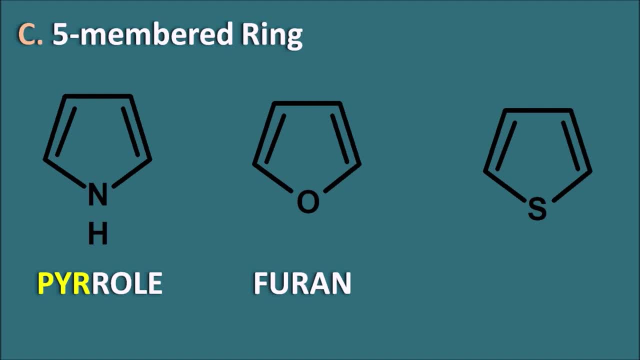 So in developing this nomenclature it is well known as a furon, So the name is going to be retained as furon. Similarly, third one is the thiophene. So these three ring systems are having a different names, like the pyrrole, furon and thiophene. Even all these are belonging to 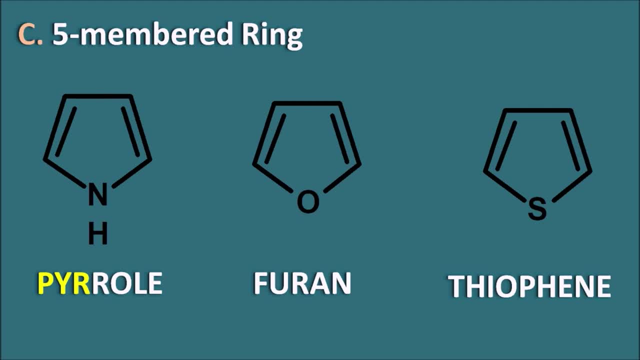 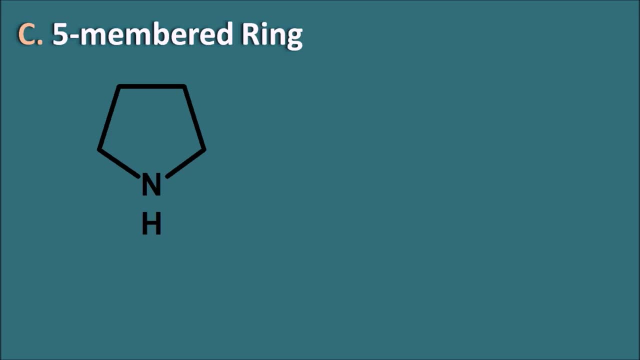 the five-membered ring systems But based on these names we can write the names of the higher heterocyclic ring systems. Now this is another example of the five-membered ring system containing the nitrogen and it is saturated. Similarly, n-ring system is having the five-membered ring system with auxin and saturated. 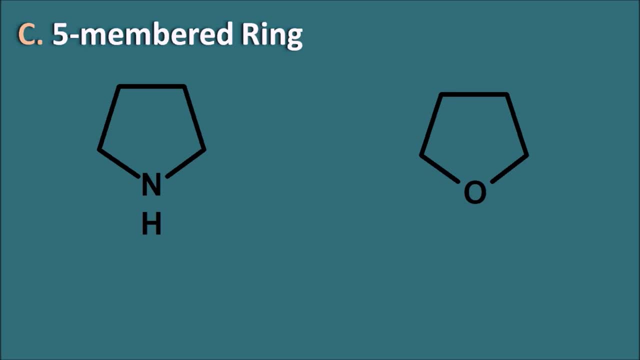 So what are the names for these ring systems? For the first one, it is a saturated form of the pyrrole, So here we can use the suffix like the oleidine. Oleidine indicates a five-membered ring system which is saturated, So pyr plus oleidine, that is the pyrroleidine, So pyrroleidine. 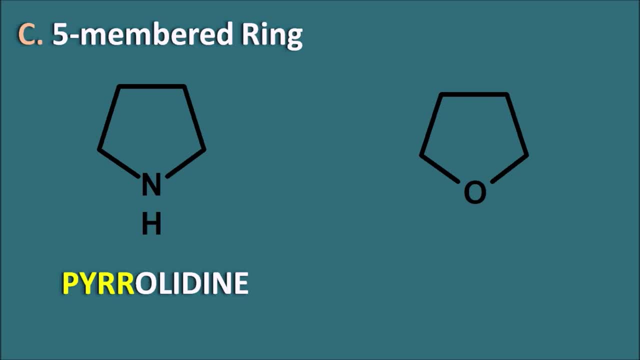 is a saturated, five-membered ring system containing nitrogen. Similarly, for the second ring, which is a saturated form of the furon, there is no specific, There is no specific prefix and suffix, But simply we can represent it as tetra-hydrofuron. 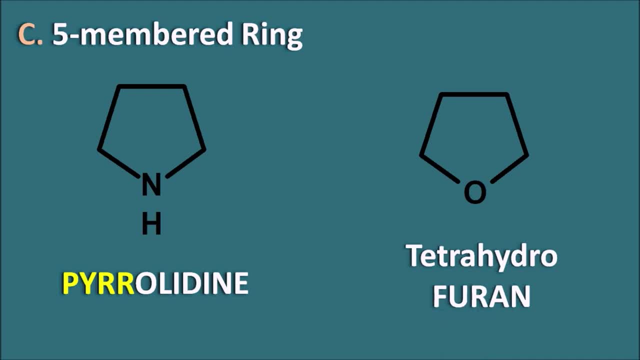 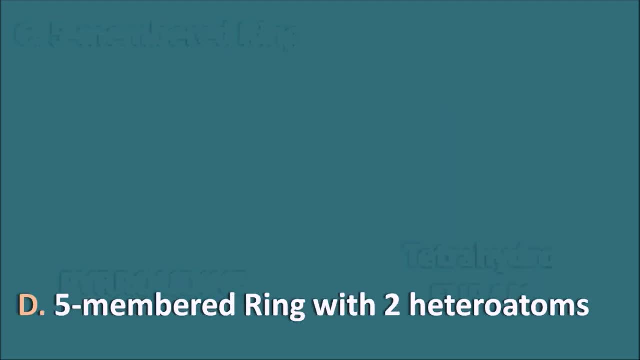 commonly known as THF. Tetra-hydrofuron is the saturated form of the furon. In this way, for few of the heterocyclic ring systems, the common name is well distributed. Next one is a five-membered ring systems with two hetero atoms. So this is one example of 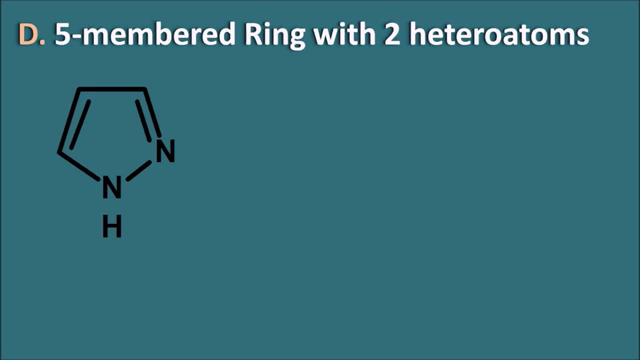 the five-membered ring system with two nitrogens as the hetero atoms. And now, what is the name of this heterocyclic ring? So, if we compare this ring system with the pyrrole, what is the difference? Pyrrole is having only one nitrogen and this is having the two nitrogens. 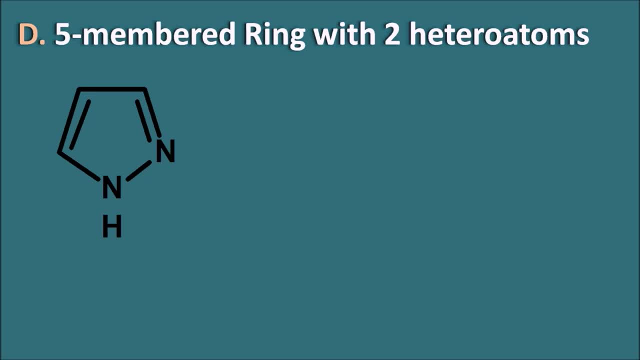 So this can be written as: pyrrole is having an extra nitrogen which can be indicated by azah, so which can be incorporated in between the name. So we can write like pyr plus azah plus ole. So pyr indicates one of the nitrogen and azah indicates another nitrogen and ole indicates 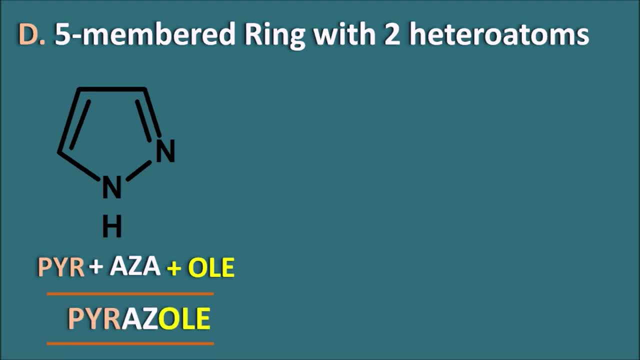 a 5 member ring system. So now this is the pyrazole. So pyrazole is the nitrogen containing 5 member ring system, with nitrogens at the first and second positions, And this is another ring system. and here, what is the name of this ring system? 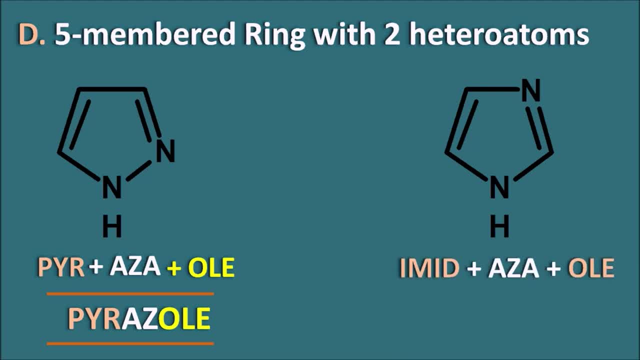 So this ring system can be written as imid plus azah plus ole. So here imid again indicates a nitrogen containing ring and azah is a extra nitrogen and ole is a 5 member ring system. So this is the imidazole. 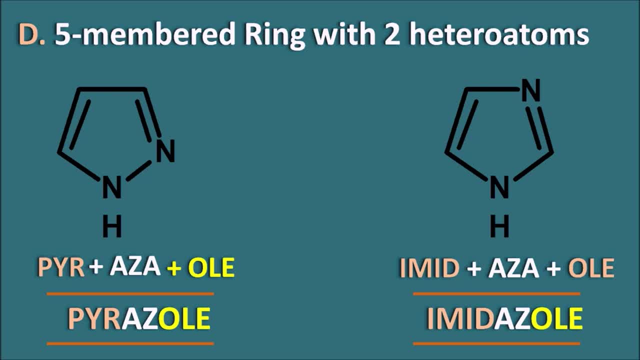 How can you remember this? pyrazole and imidazole- We may be confused with that. keeping the help of Ondうん cah Mixology. drop down those numbers because we did not define mu the initials earlier. So what will be essentially we are going to do now is thely unique. so, like in pyr isol. 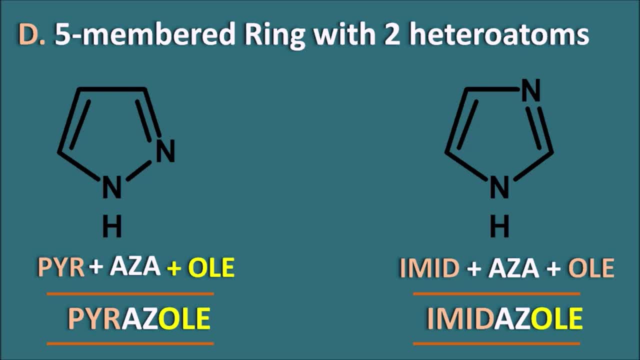 is having the nitrogen, that the first and second position, or 1st and 3rd. It can be easily remembered that this imid indicates here where letter M is there. M indicates like the meta position, that means the third position, Just like the aromatic ring system, ortho meta para. 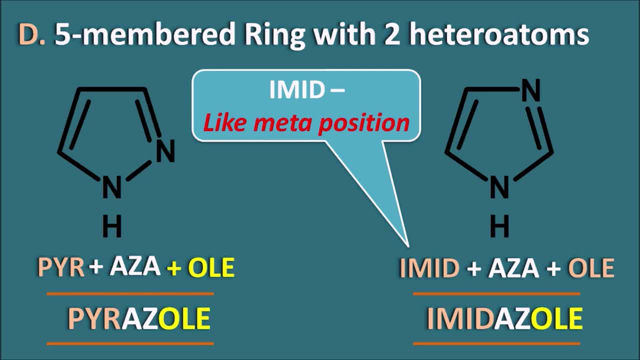 So the M indicates here the meta position. that means the second nitrogen is present at the meta position to the 1st one. that is a third position. So whenever M is there, then indicates the third position. Why is the second person present? it is because the second nitrogen, Chris, is present in the 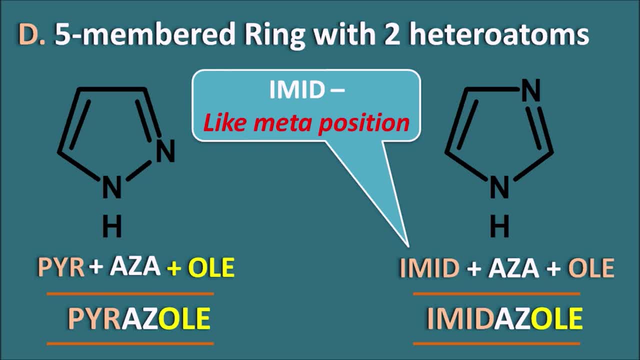 third position. so imidazole is having the second, nitrogen at the third position. in this way we can easily differentiate the pyrazol and imidazole. pyrazol is one two, imidazole is one three. similarly, another ring system is having oxygen and nitrogen. what is this? so here the oxygen is. 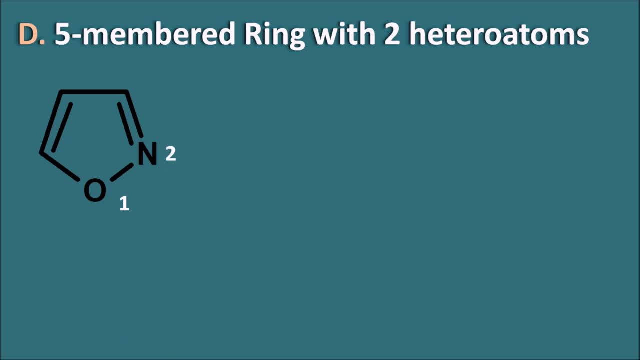 present at the first position and nitrogen is present at the second position. always we have to give the preference to the oxygen, then to the nitrogen. so here the oxygen and nitrogen are present at the first and second position, and oxygen can be indicated by oxa and nitrogen as 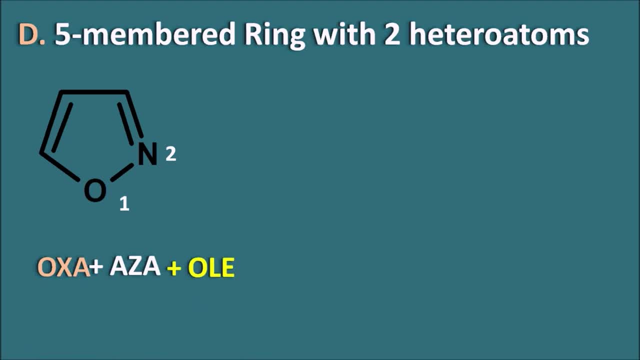 asa and it is a five member ring system. all so this is an oxazole. the hetero atoms are present at the first and second position, so this can be written as one, two oxazole. so this one two oxazole is commonly known as isoxazole. so here you have to remember that isoxazole the iso indicates first. 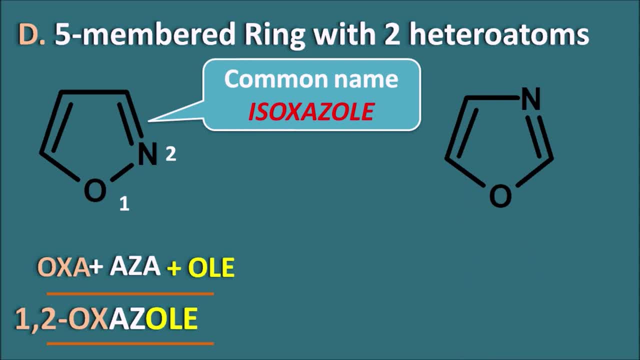 and second position. if we see another related ring like this now here, oxygen is present at the first position whereas nitrogen is present at the third position. so this is again oxa plus aza plus vol, with the first and third positions having oxygen and nitrogen. so this is the one three.